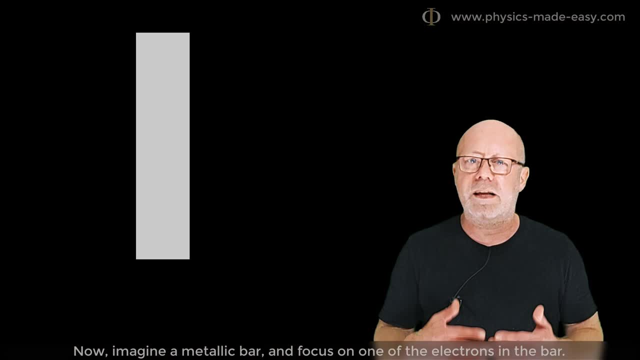 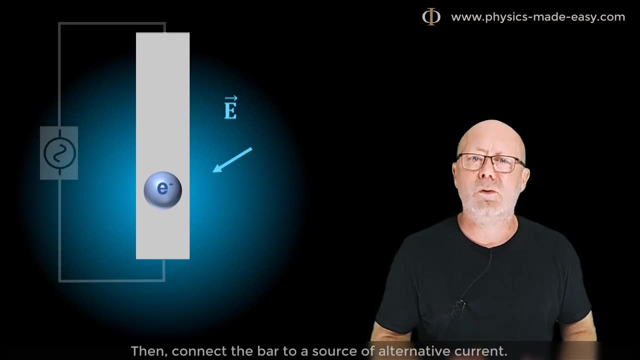 Now imagine a metallic bar and focus on one of the electrons in the bar. This electron creates an electric field around it. Then connect the bar to a source of alternative current. The electron will move back and forth in the bar with the current. 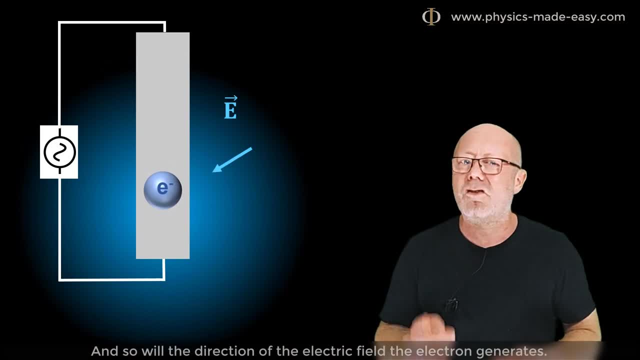 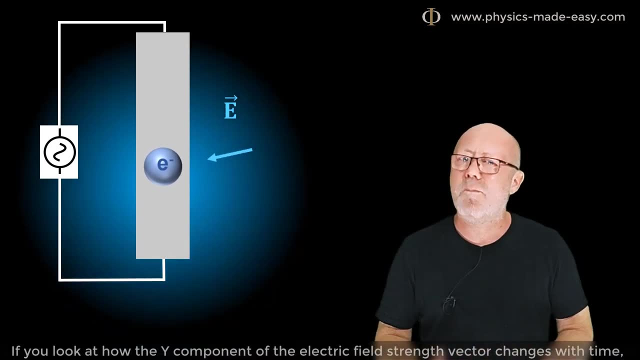 It will oscillate, And so will the data, And so will the direction of the electric field the electron generates. This idea is a key point If you look at how the y-component of the electric field strength vector changes with time. it is oscillating. 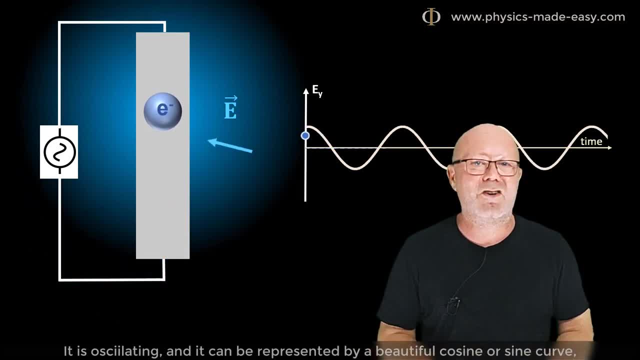 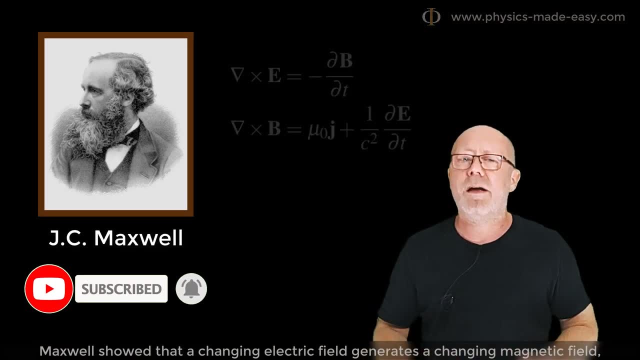 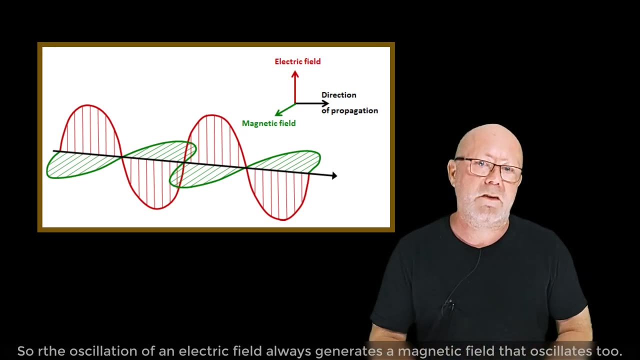 And it can be represented by a beautiful cosine or sine curve. In the second part of the 19th century, Maxwell showed that a changing electric field generates a changing magnetic field, and vice versa. So the oscillation of an electric field always generates a magnetic field that oscillates too. 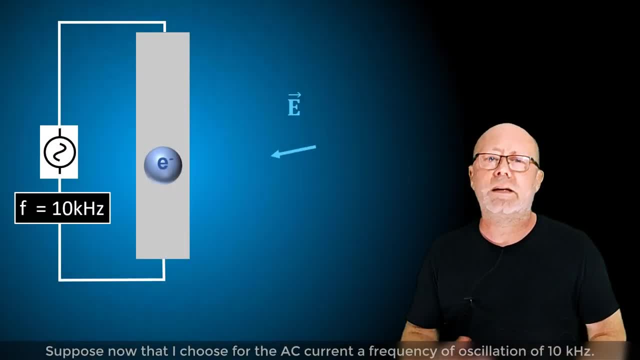 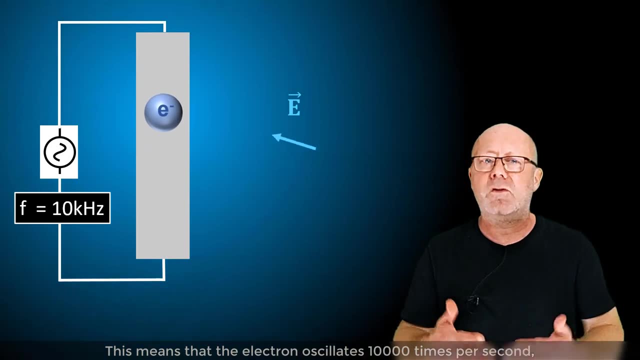 Let's go back to our electron. Suppose now that I choose for the alternative current a frequency of oscillation of 10 kilohertz. This means that the electron oscillates 10,000 times per second, And so does the electric field it generates, as well as the induced magnetic field. 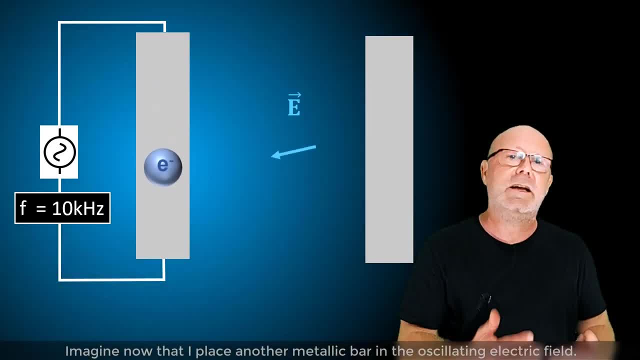 Imagine now that I place another metallic bar in the oscillating electric field. The electrons in this bar will feel an oscillating force. Yes, they are in an electric field, so they feel a force. They will also feel an oscillating force. Yes, they are in an electric field, so they feel a force. 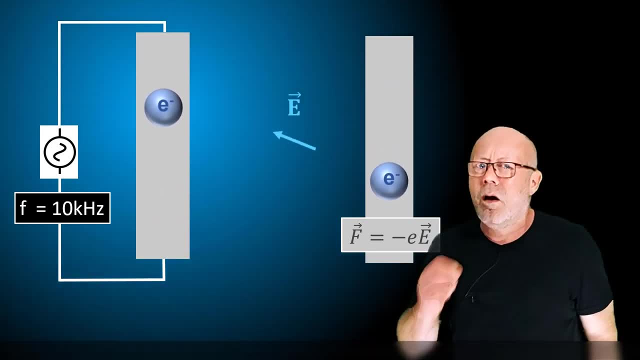 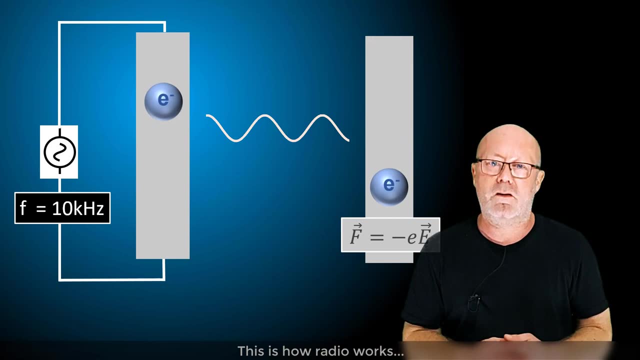 Yes, they are in an electric field, so they feel a force. They will start to oscillate too. What we did here is we transmitted a signal through space. This is how radio works. Yeah, we have two antennas. The first bar is emitting the signal. 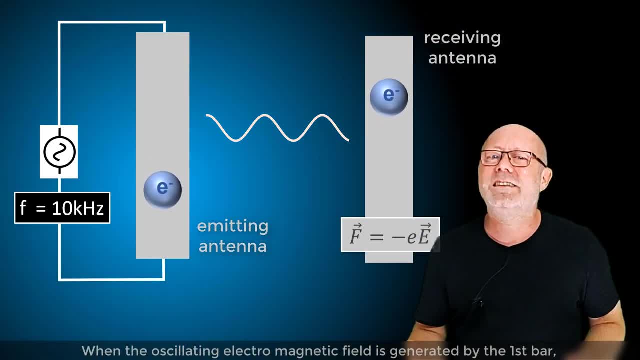 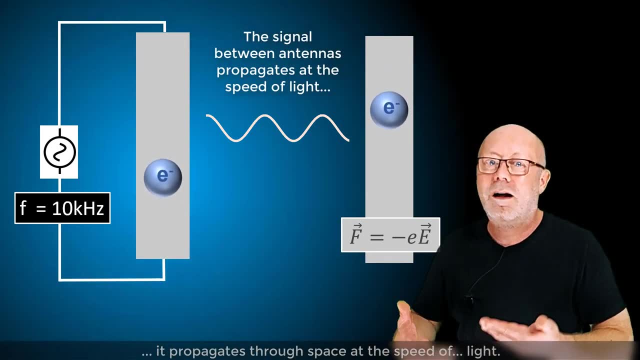 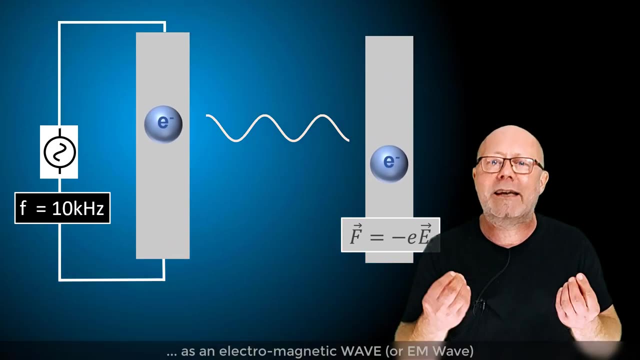 The second bar is receiving the signal. When the oscillating electromagnetic field is generated by the first bar, it propagates through space at the speed of light. Yeah, the oscillating electromagnetic field is what we refer as an electromagnetic wave or EM wave. 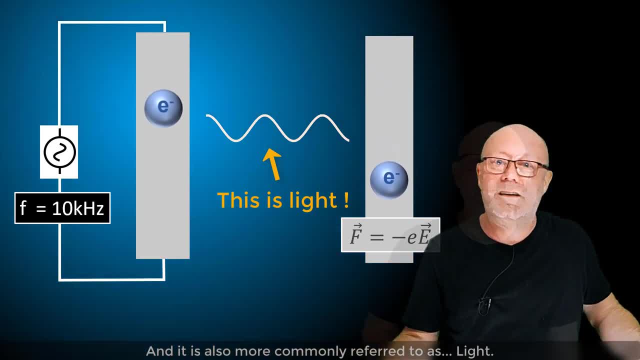 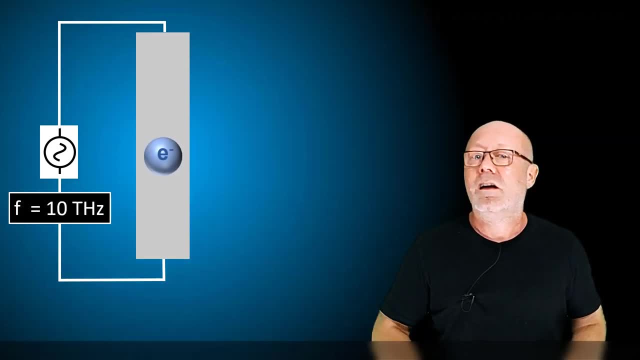 And it is also more commonly referred as light. For example, let's increase the frequency of the alternative current up to 10 trillion hertz. The electron in the bar will oscillate at 10 trillion hertz, and so will the electric field it generates.